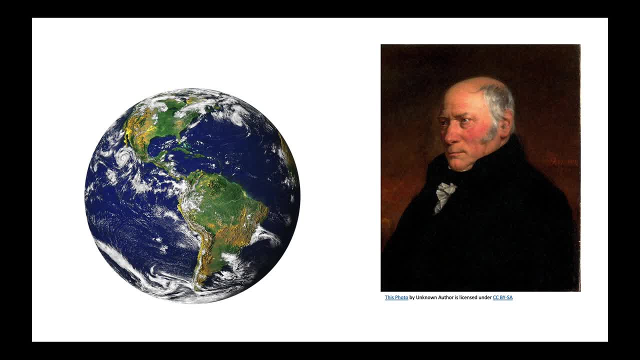 layers are at the top. By the early 1800s, people were beginning to get the idea that Earth was perhaps a little older than originally thought. One of these people was William Strata Smith. Smith worked for a coal mining and canal digging company and he was generally 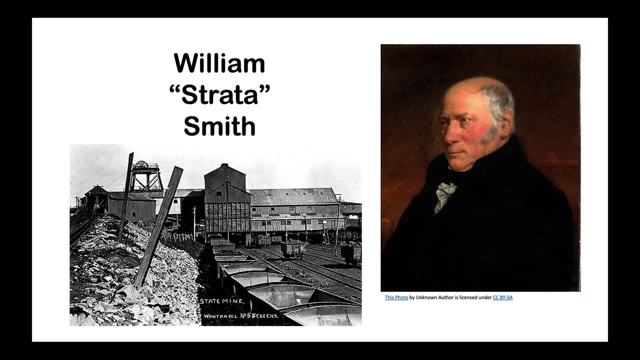 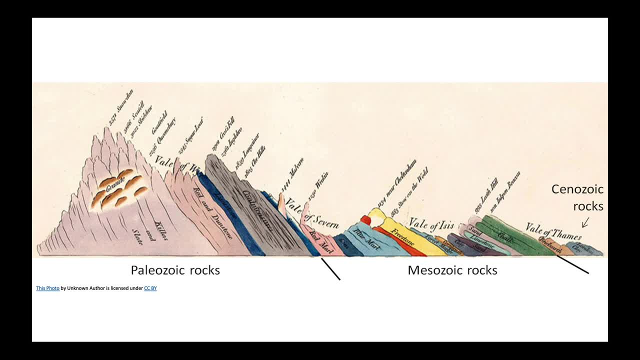 observant and a curious guy with a really cool nickname too. In his work all over England he noticed the same rock layers, such as the layers he called chalk and lulius, could be found all over England and in the same order. Smith also noticed that each of the layers 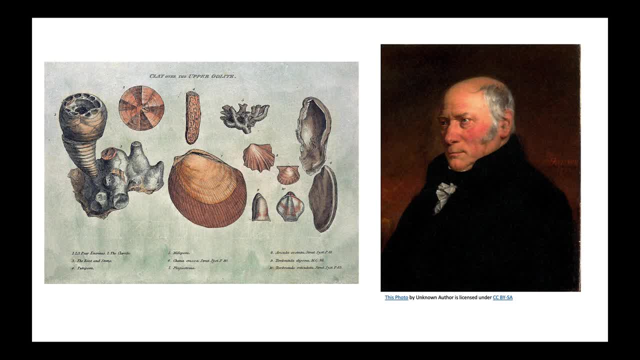 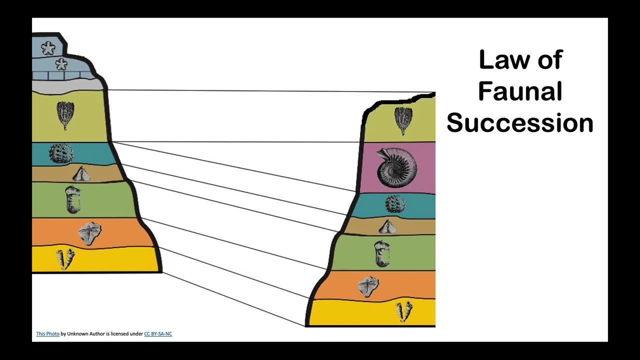 contained its own special set of fossils, Distinct from the fossils found in other layers. Smith figured that fossils must also be like rock layers: Older fossils are found in deeper layers and newer fossils are deposited on top of the older fossils. Strata Smith called the way that layers of fossils stacked. 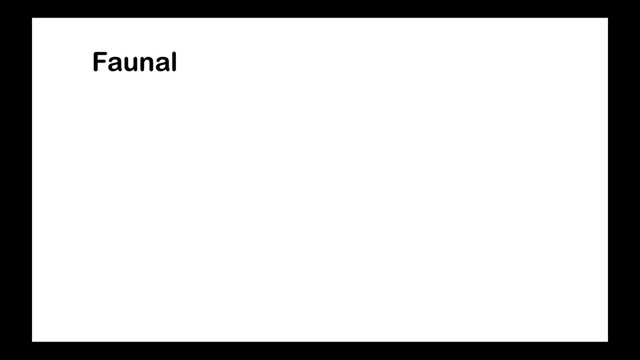 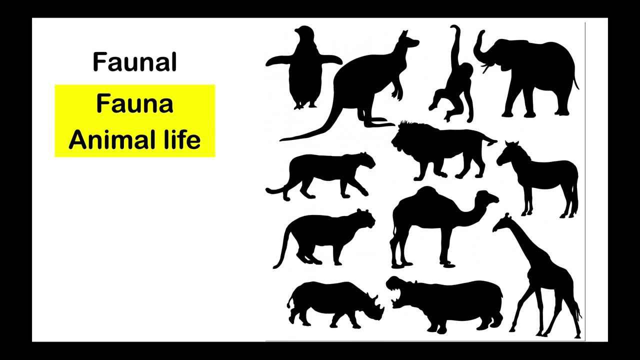 up the law of faunal succession. Now, faunal is a word that comes from fauna, and fauna just means animal life. Sometimes Smith's law is also called the law of fossilization, Fossil succession. Because of Steno's and Smith's work, we know that rock can be found. 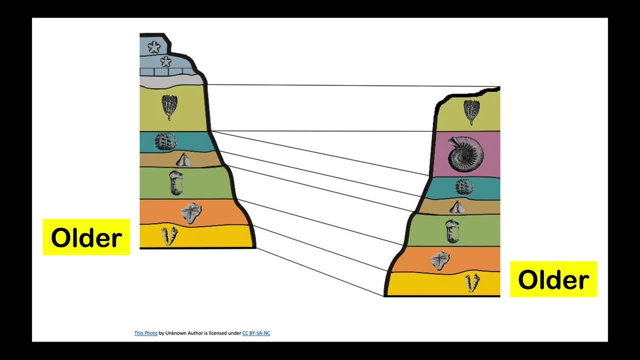 in layers. The layers are stacked, with the oldest layer at the bottom and the newer layers on top. The fossils found in the layers are stacked in order of age as well: Older fossils on the bottom, younger fossils on the top And fossils found in the same rock. 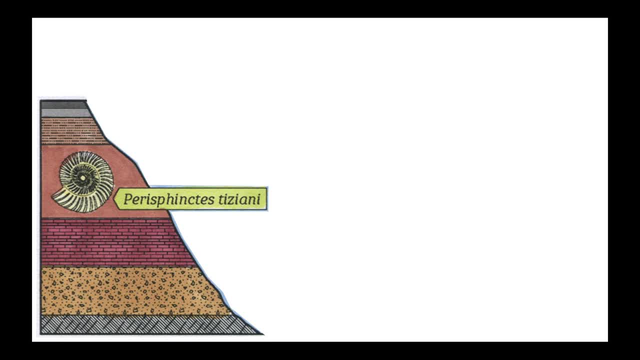 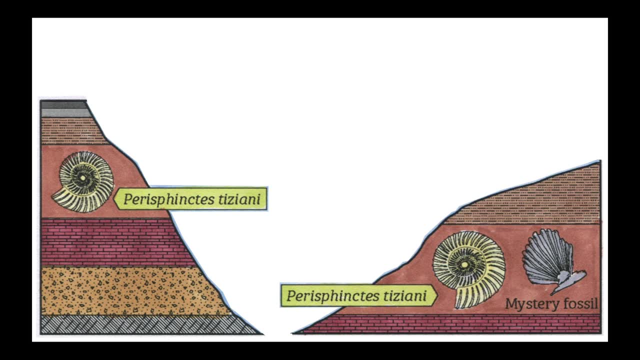 layer are approximately the same age. So if you find a specific type of ammonite fossil in a layer in one location and the same type of fossil in the same layer, then you're sure that the two fossils are about the same age. Not only that, but the rock layers, the 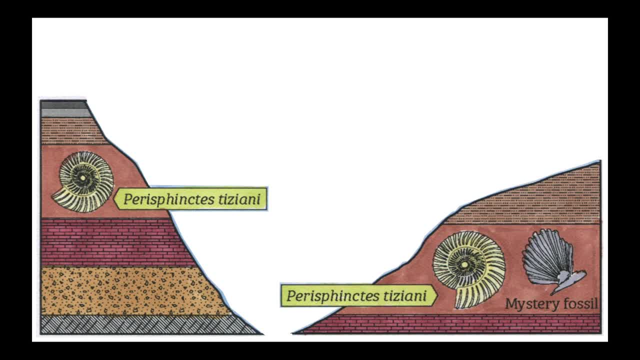 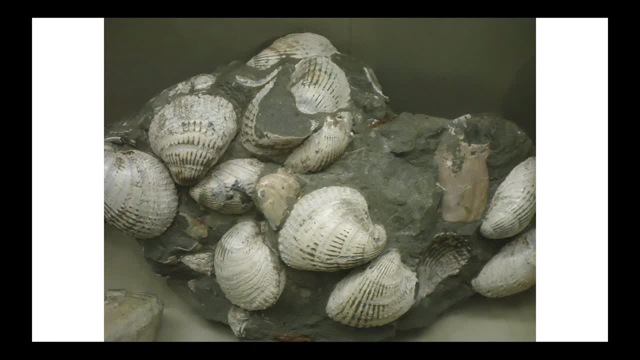 fossils are found in are also about the same age. It's pretty obvious that two or more fossils of the same species found side by side in the same rock layer are roughly the same age, But sometimes rock layers are interrupted. You might find a specific type of trilobite. 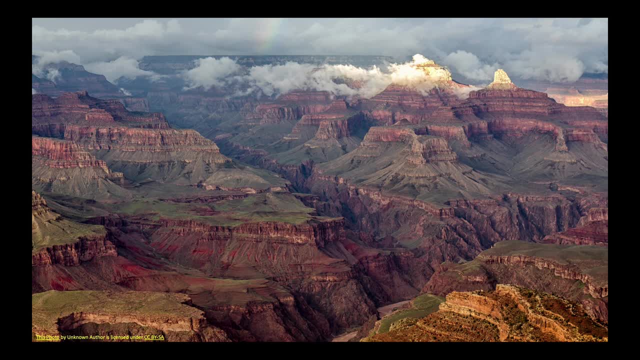 fossil in the bright angel shale in the Grand Canyon and the same type of fossil in the same layer on the other side of the canyon. Even though the fossils are far apart, they are still the same species in the same layer, so they're roughly the same age You can find. 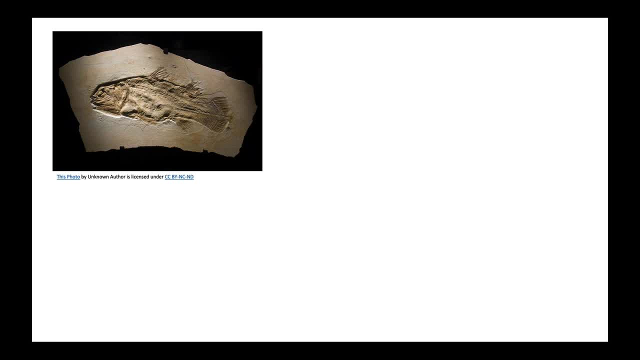 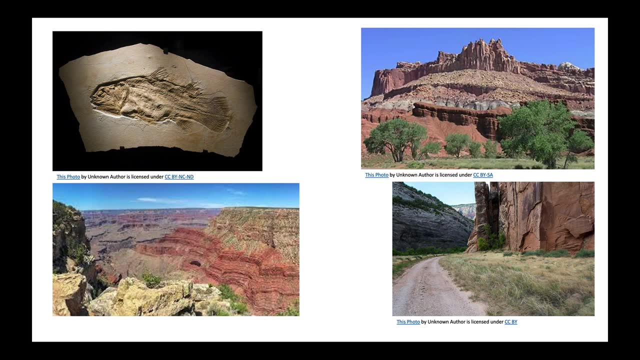 fossils of similar fish species in the Moonkopi Formation, in the Grand Canyon, in Capitol Reef National Park and in Dinosaur National Monument. These places are not all that close together but the fossils are found in the same rock layer, so we know the fossils are. 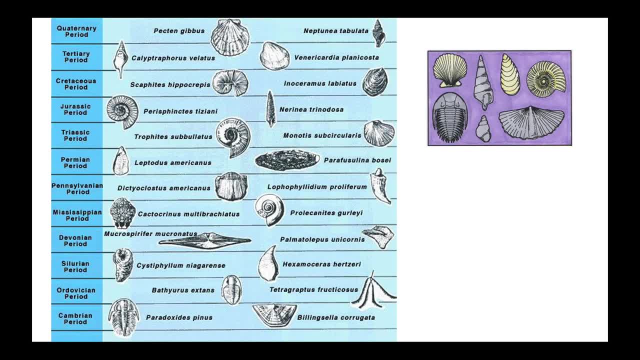 of the same age. Fossil succession helps us determine the age of rocks and fossils, and there are certain fossils that help determine the age of other fossils and rock found in the same sedimentary layer. These are called index fossils. Here are some examples of index fossils- Not all. 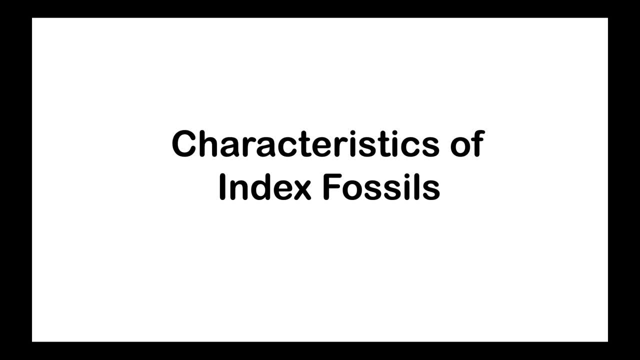 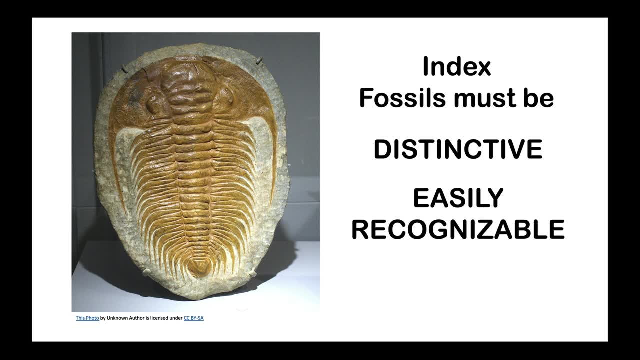 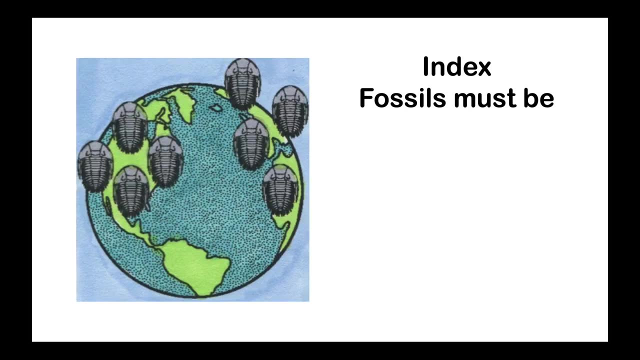 fossils are index fossils, though These are the characteristics of index fossils. Index fossils must be distinctive and easily recognizable. That's a pretty easy trilobite to recognize. It's pretty distinctive, but that's weird, Your little trilobite head. 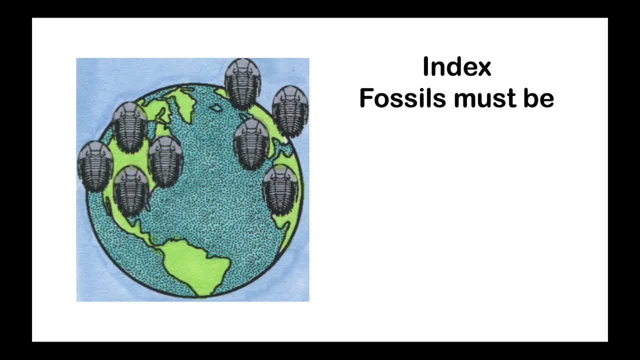 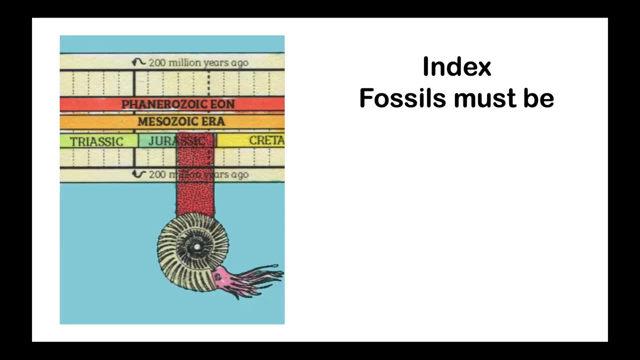 Index fossils must be globally widespread, That is to say found in a lot of places all over the globe. Index fossils must be abundant. Index fossils must also be organisms that became extinct fairly quickly. This is helpful because finding fossils that lived only during a very precise time helps pinpoint the age. 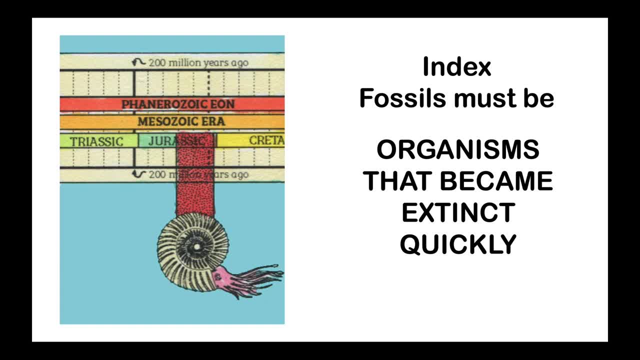 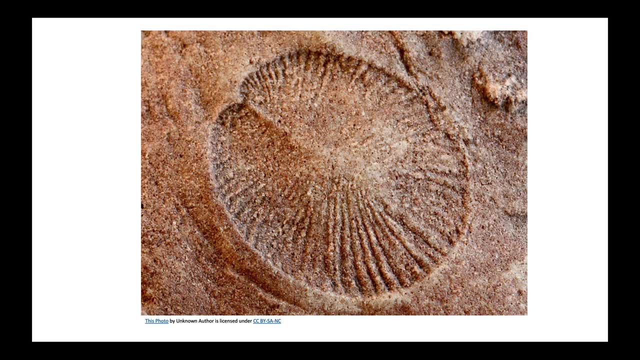 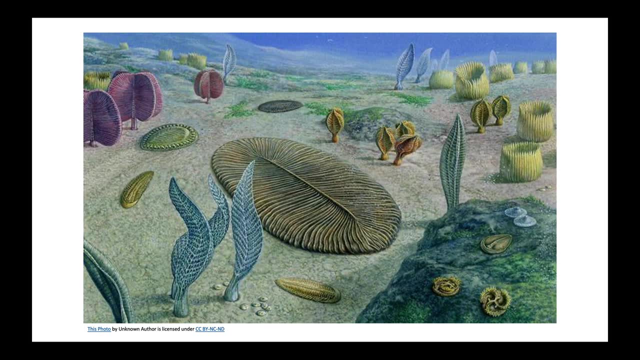 of anything else that lived at the same time and whose remains are found in the same rock layer. For example, this incredible Ediacaran fossil from the Precambrian super-eon was made from soft-bodied creatures that were abundant about 600 million years ago. But because their bodies 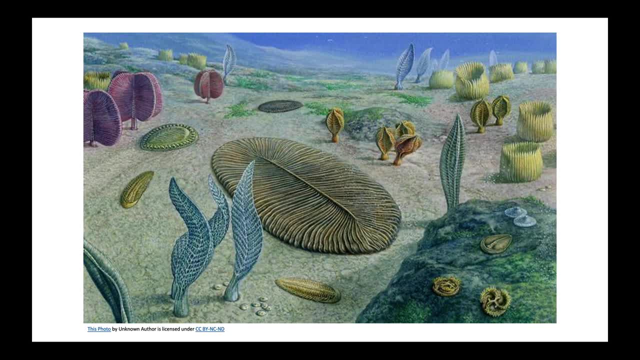 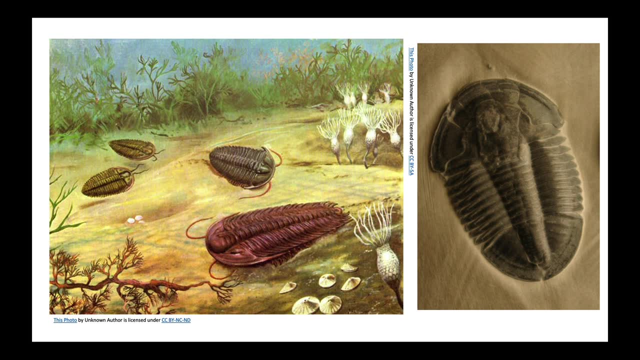 were soft and jelly-like. we don't find their fossilized remains very often today. In fact, they're very rare to find as fossils. Did you notice that many index fossils are from animals that lived in the ocean? It's no coincidence. 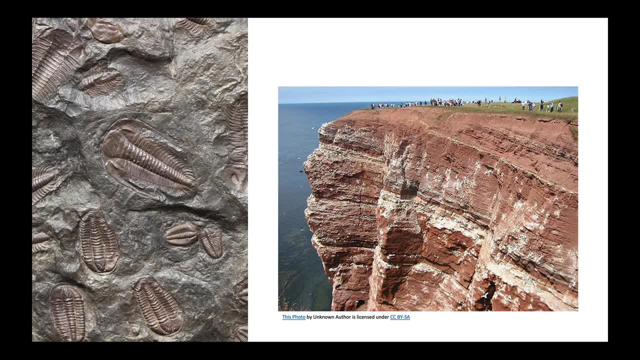 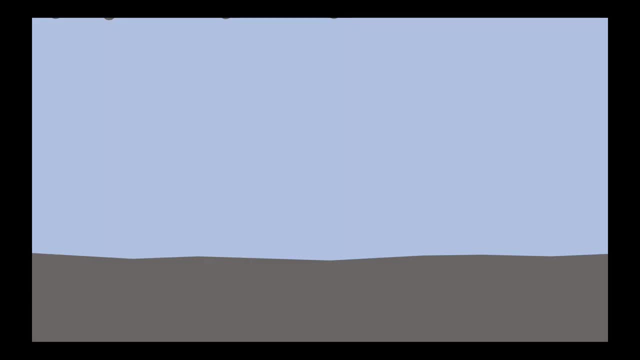 Fossils are almost always found in the sea. They're very rare to find in the ocean. They're always found in sedimentary rock, and sediment is carried by water In the ocean. sediment sinks down to the bottom. Dead things in the ocean also sink to the bottom, so it's way. 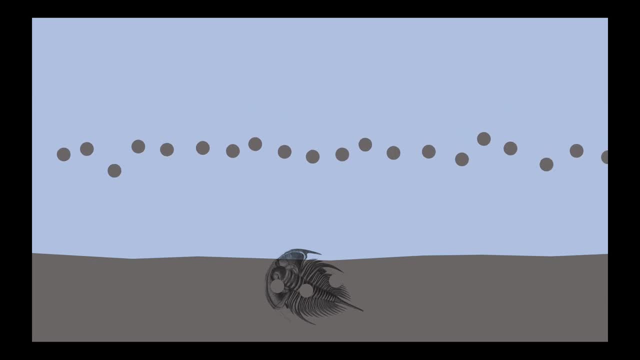 more likely that the remains of something dead will be preserved in sedimentary rock in the ocean than on land. Additionally, many animals that live in the ocean reproduce by casting their eggs into the water. Ocean currents pick up these floating eggs and larvae and carry them all over the